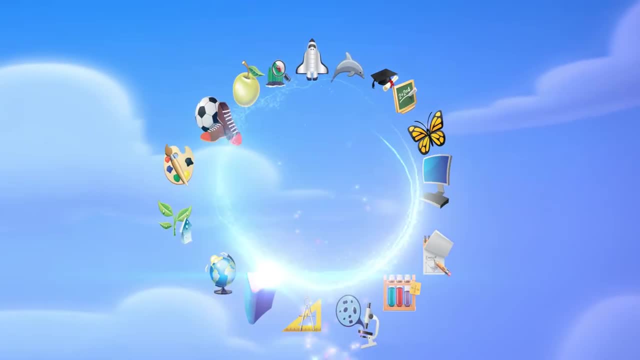 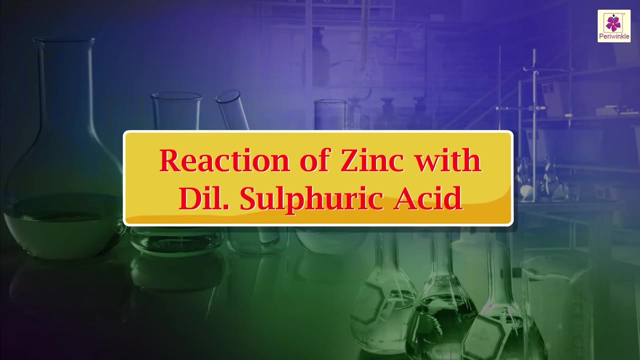 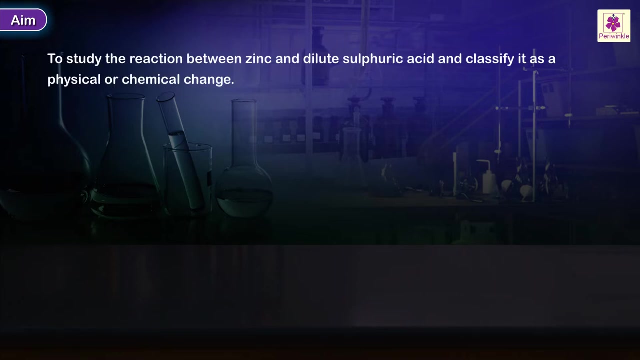 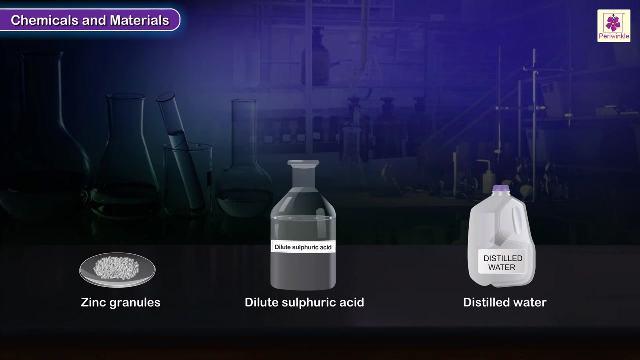 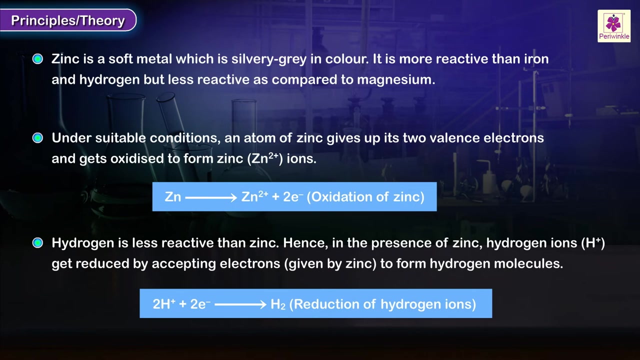 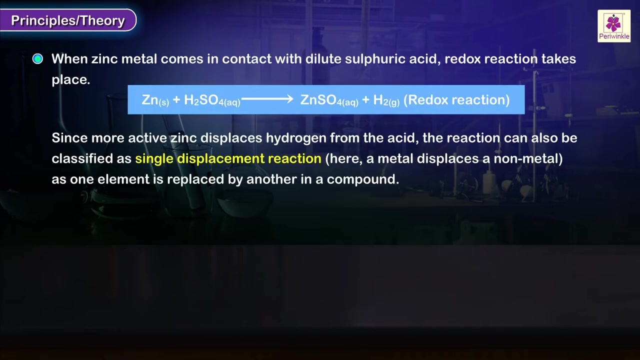 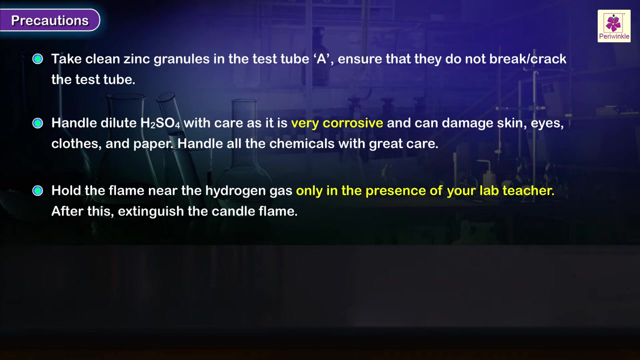 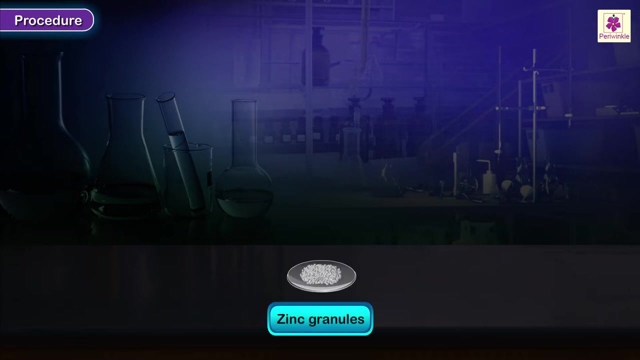 Reaction of Zinc with Dilute Sulfuric Acid. Aim To study the reaction between zinc and dilute sulfuric acid and classify it as a physical or chemical change. Apparatus, Chemicals and Materials. Principles, Theory, Precautions. Procedure: Thoroughly wash the given zinc granules and take a few of them in a hard glass test tube labeled A. 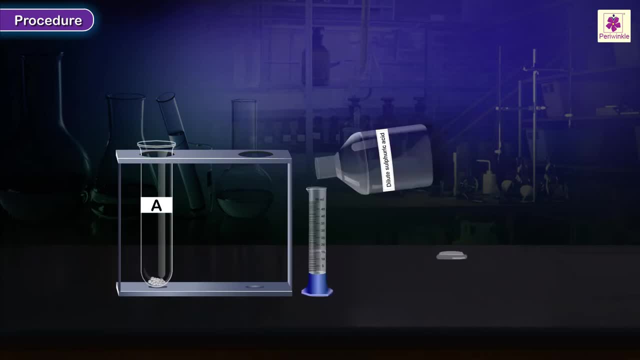 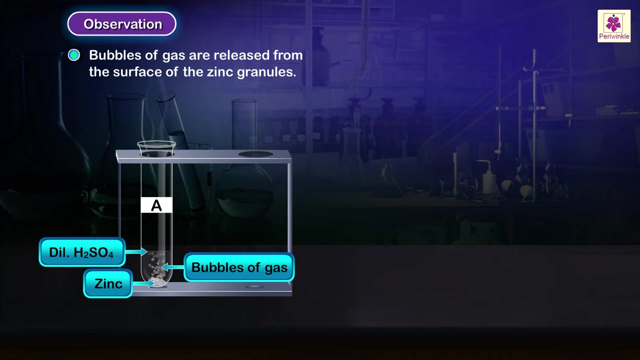 Carefully add about 10 to 15 milliliters of dilute sulfuric acid to it. Observations: Bubbles of gas are released from the surface of the zinc Zinc granules. Inference: Zinc reacts with dilute sulfuric acid. 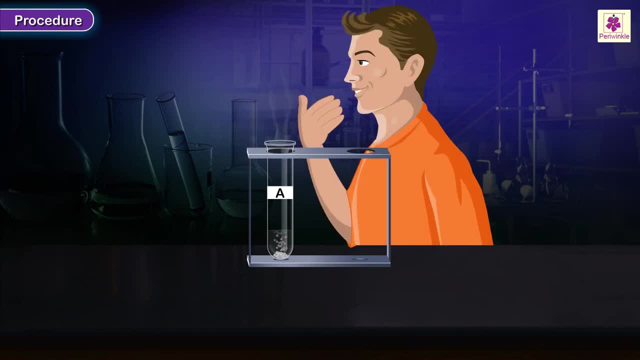 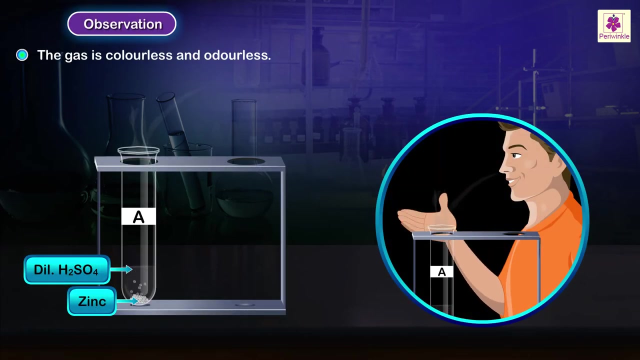 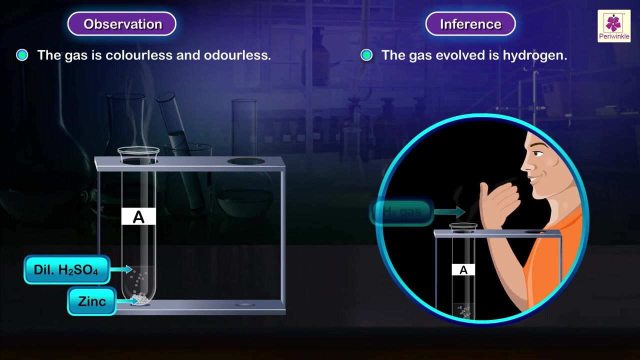 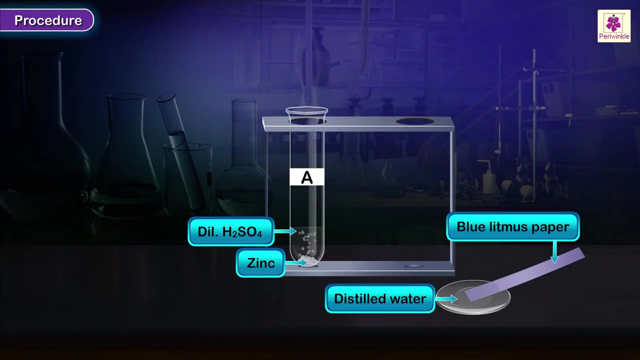 Procedure: Fan the gas evolved gently towards your nose with your hand and note the smell of the gas. Observations: The gas is colorless and odorless. Inference: The gas evolved is hydrogen. Procedure: When the gas evolves in the test tube, hold blue and red litmus papers moistened with distilled water at its mouth. 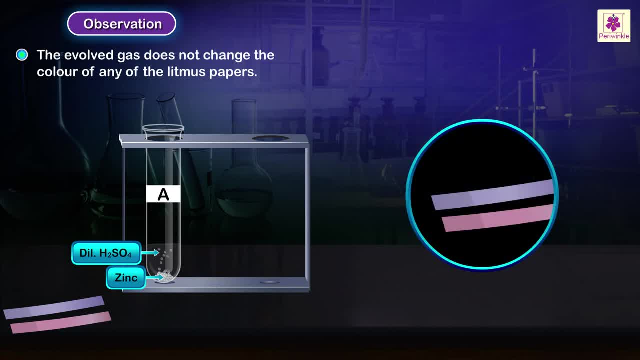 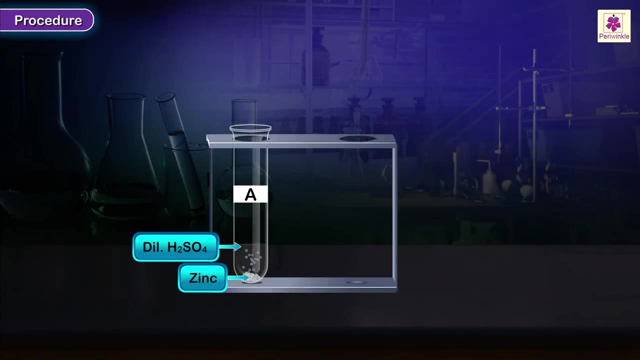 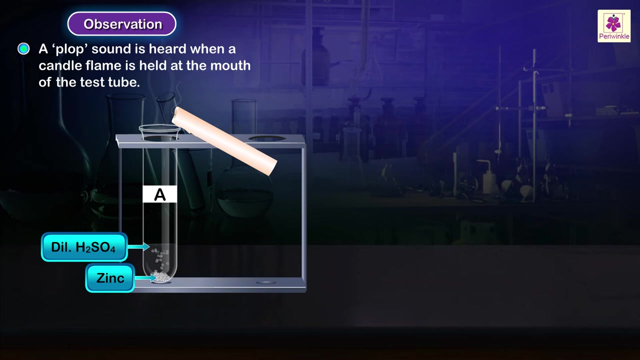 Observation: The evolved gas does not change the color of any of the litmus papers. Inference: The gas is neutral. Procedure: Hold the flame of a burning candle at its mouth and observe the effect. Observation: A clop sound is heard when a candle flame is held at the mouth of the test tube.